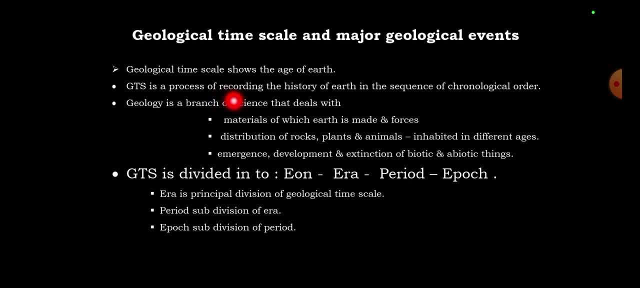 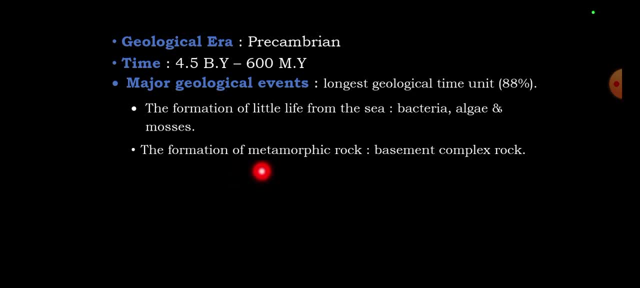 So Geological Timescale is a process of recording the history of Earth in the sequence of chronological order. So Geological Timescale is a process of recording the history of Earth in the sequence of chronological order. So pre-Cambrian is the longest geological time unit. 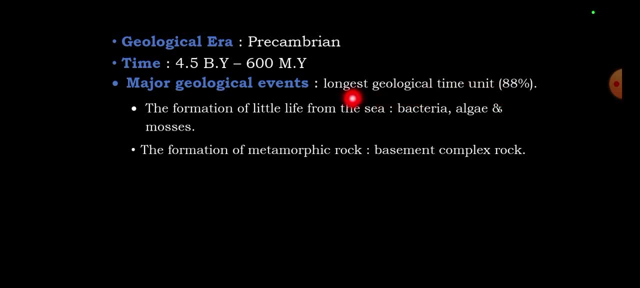 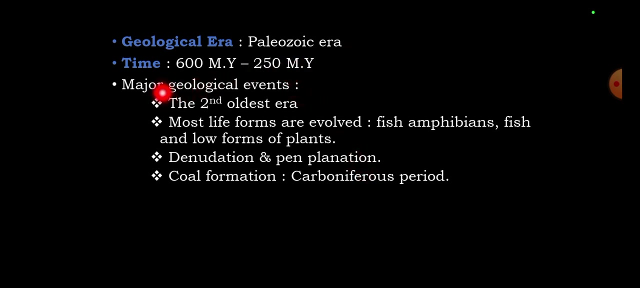 So pre-Cambrian is the longest geological time unit. This unit shows us that pre-Cambrian is the almost 10 year cycle of life. Also, pre-Cambrian is the course of time period before it is called gory. 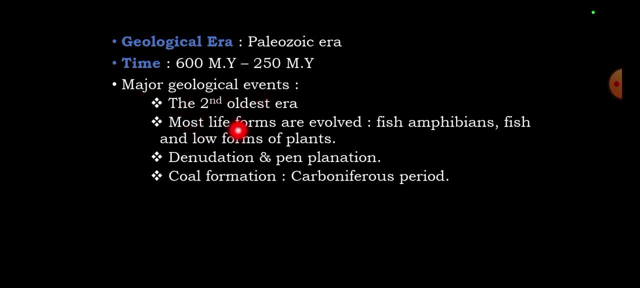 With this MSS is the small difference between MSS and Pre-Cambrian. Before MSS succeeded MSS didn't? Some have said that before MSS There were no more known evolutions like MSs. 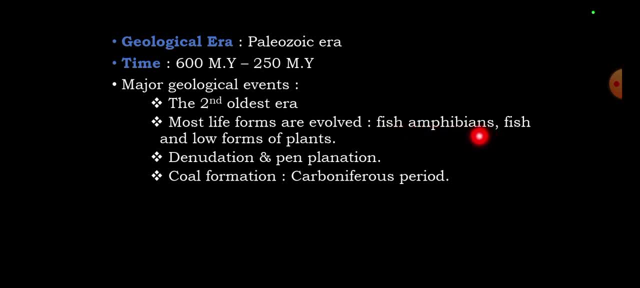 Like no kickể West winds or lower seas, Like no kickể West winds or lower seas. fish amphibians is in doom law forms of plant me, but the federal but casino malatino deludation and pain plan is in denudation, mallet erosion and now. 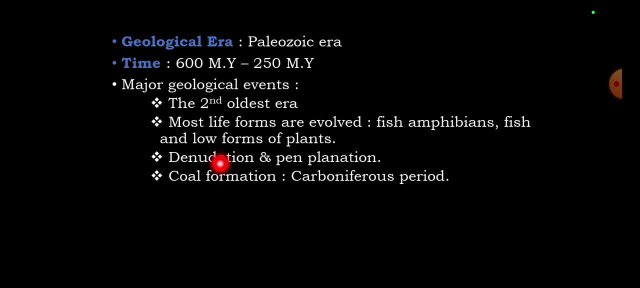 weathering, marital erosion, malatransporting of eroded material. it is her a sharon, a garage boat. hot boss. you said you erosion benefits that bow wiener berber dotat possible said erosion in parallel, wiener weathering. until you can add it this, high high lena the brodomic. 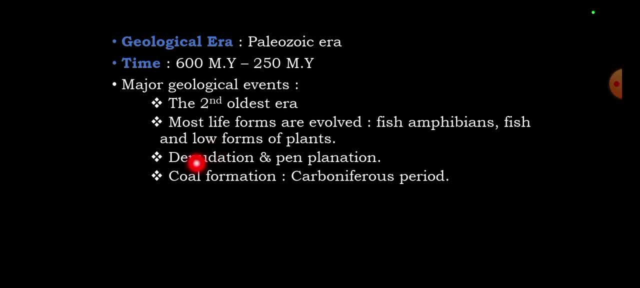 Kasaba, rodent analysis about secure weathering, give us a little denudation, malatino, lowering of land surface and high mountain with a second, a terrarium massive for a wiener with a medium massive classic here, denudation in balance, there's a denudation, mallet, lowering of land surface, mallet, no pain. 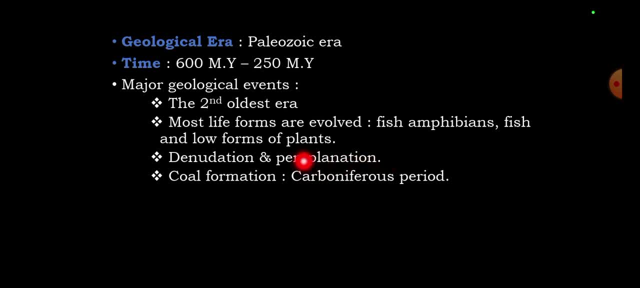 planations in the lagoon medium, my own sifra out plain area, malatino. so stenia call formation. so let's see the sustenance come to the formation of call. you didn't like it a little better. but get a nomadic period, ooh, mini ballad carboniferous period, a ballad arrow. 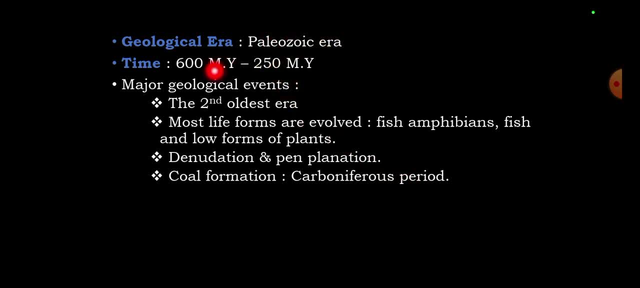 palazzo, a key ballad. lazy palazzo, kira, because it is moscow, let me know how much. I mean. I'm at a log. is you know? when I went into it is a second oldest. let's hang out. I don't give a ballad monitor. most life forms busy with. 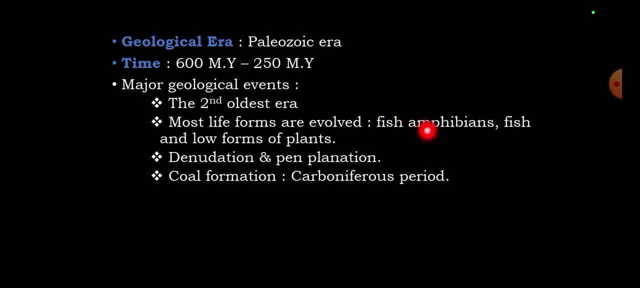 stuff at the rabbit room, amphibians, but the amphibians. but I'm in direction to start with you, to better button. the missile is a unit, yes, a zero, which, and do it right, in it you encourage area which the federal button doom. it, allow you a net low forms of plant. 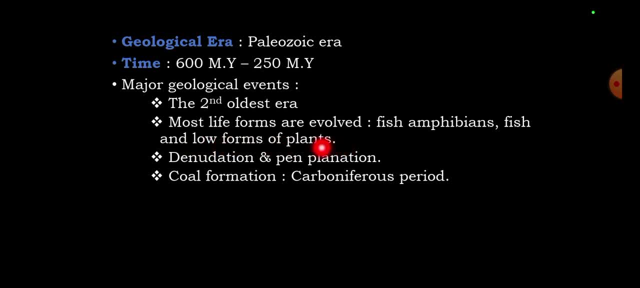 millennium drachma missile. a friend in this unit is what you the federal, but getting a minute and you get a nation pain planation. call formation in the cut during carbon first period. you will. I'm not at home but hosting in the thumbnail geological era, may so zoic era ballad. 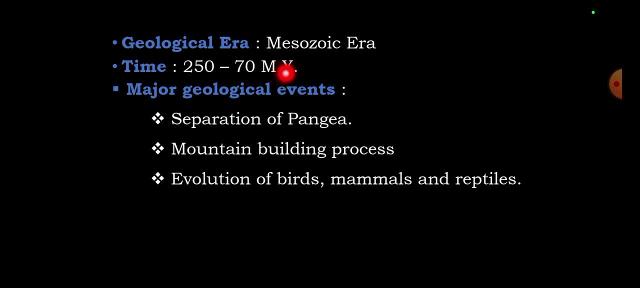 beg raises of the ortion of beyond subpar 나올 basha. separations of не been sitting inподres served trouble. separation of the issues are perched on us because are born asım and the number of plans for destruction diabetes persists when workouts come to. incarnation happ engine. yeah, we're not having such a bad time right now, we're either doing it. so Sugar our backbones. What about your facility in North America? Nam epic request. Asian 눌러 Vargas, America, Because zugワ due, do not resist the. 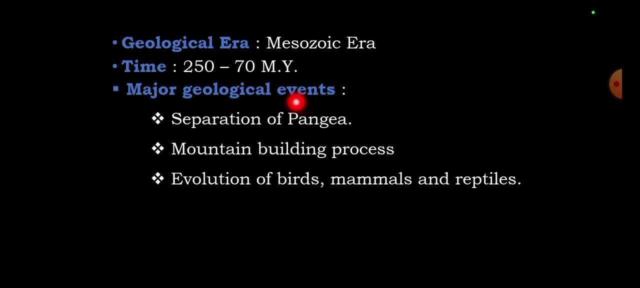 The other one's evolution of birds, mammals and reptiles. The other one, Pyrapoidosis Moozلةus, can also grow these plants by growing baind Greenwegen, the iota plant and Highland mullet too, and they grow co- 플�. oak. 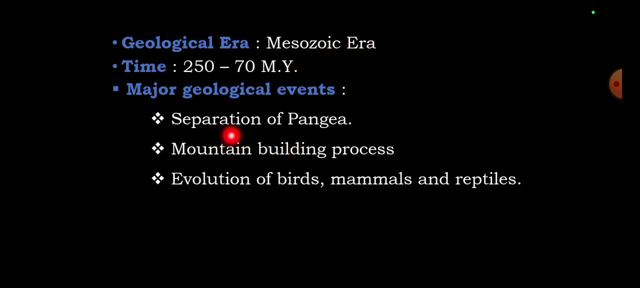 Why? Beacuse they're actually reachable. In fact, them grow in arid areas like organized trash. So the formation of separation of pangaea, mountain building process, evolution of birds, mammals, reptiles and the formation of flowering plants during Mesozoic Era. 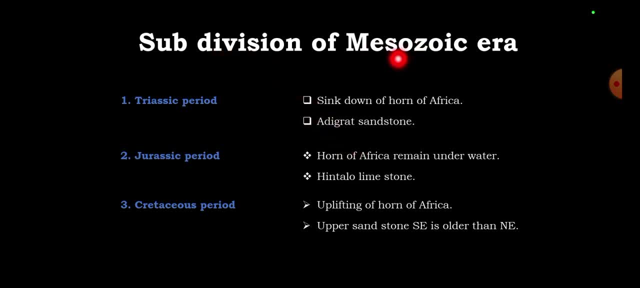 Mesozoic Era is classified into two. Mesozoic Era, as you can see, is called the Jurassic Period or Jurassic, as you can see, the Cretaceous Period. Jurassic Period, as you see, is the Sink-down of the Horn of Africa. 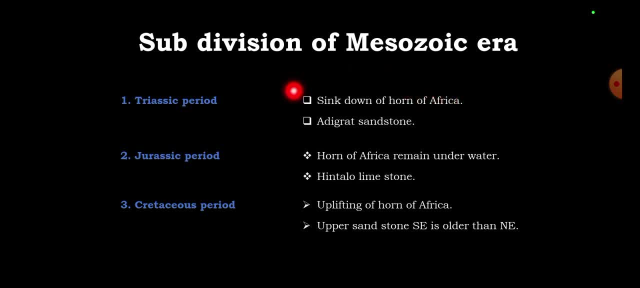 Horn of Africa is the name of all the contry with a golden title. The Horn of Africa is the name of Ethiopia, Eritrea, Somalia and Gebotena. So when you look at the position of the Horn of Africa, you have two golden titles. 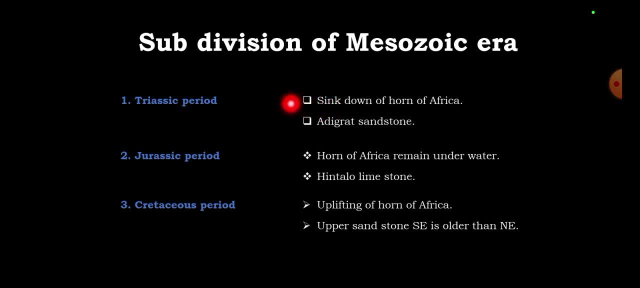 So all of the three местоings are named after the Horn of Africa. that's why it's called the Jurassic, The. I'm going to tell you a story about a man who was born in Africa, and he was born in the year of the tiger. 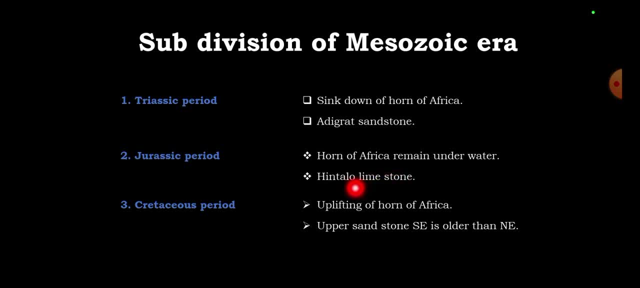 He was born in the year of the tiger, and he was born in the year of the tiger and he was born in the year of the tiger. So I'll tell you about a man named Cretaceous. Cretaceous was born in multiple countries in Africa, such as Ethiopia, three-world 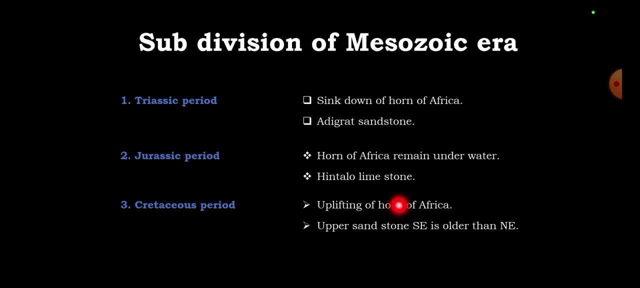 Jaebutina and Somalia, And he was born in the year of the bear And he moved to the south of Africa Because he was born in the year of the tiger. he could not make a emperor And that was written there on a happening stone. 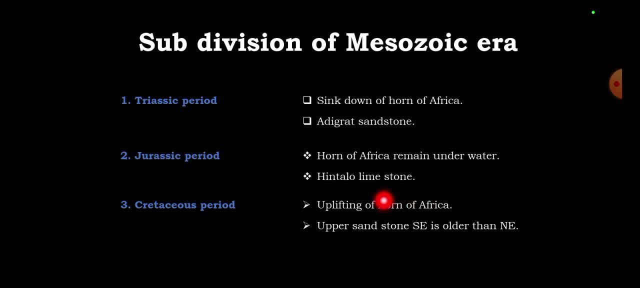 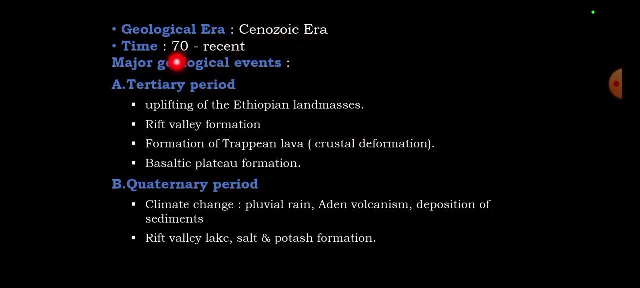 South East is the northern part of the country. North East is the northern part of the country, So the South East part is old, North East is young. The second area is the Cenozoic area. This area is called the Cenozoic area. 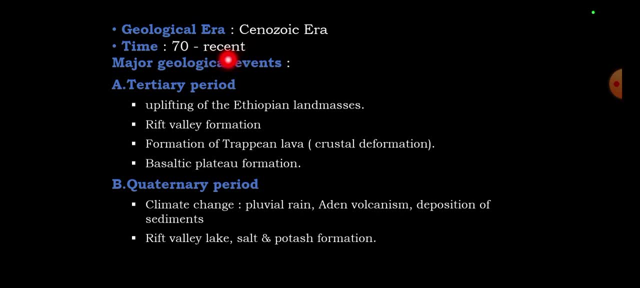 It is the Cenozoic area. It is the Cenozoic area. It is says that the end of the extension period is called the Cenozoic and Quaternary period. When you are thinking of zien 전 at the apply of schwierings in Ethiopia. 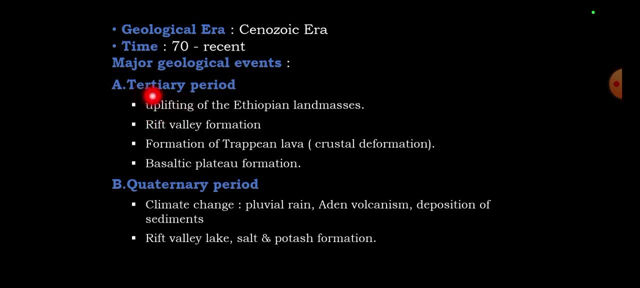 the top of Ethiopia. you think of Cenozoic Ad alla. when you think of the April formation, it is called the Cenozoic period. From the, etc. I can see that the rain is coming, As if rain is not a big problem. 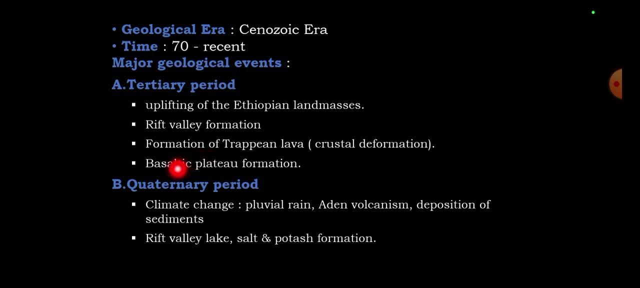 It is just a small amount of rain. It is because of the basaltic plate formation. It is the base of the earth. The earth is formed by the basaltic plate. The basaltic plate is the foundation of the earth and it is also a source of rain. 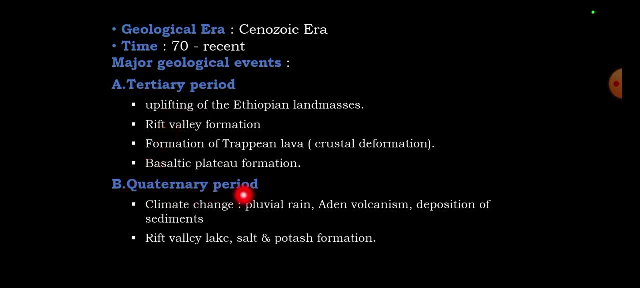 that is why the rain is coming. The weather is also a good thing. It is a good climate weather. It is a good weather, But the weather is not great. It is usually heavy rain is the rain that is in the form of the Pluvian rain. 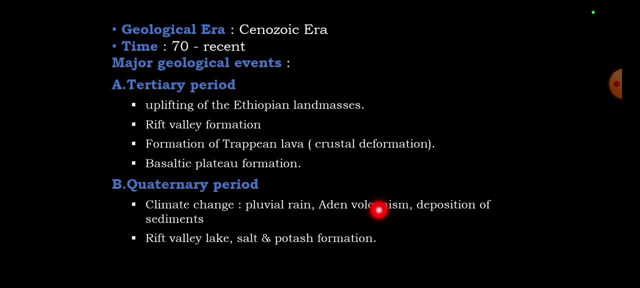 So the Pluvian rain is the volcanic deposition of sediment in the region. So the way that the water flows is the way that the water flows between the soil and the soil. For example, in Ethiopia, the water that flows through the soil is different from the water. 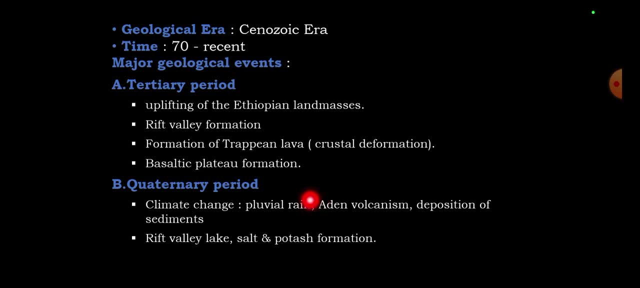 that flows through the soil in the area, So the water that flows through the soil is not repaired. Let's look at the situation in Ethiopia, For example. there are things that are being done for the environment, For example. there are things that are 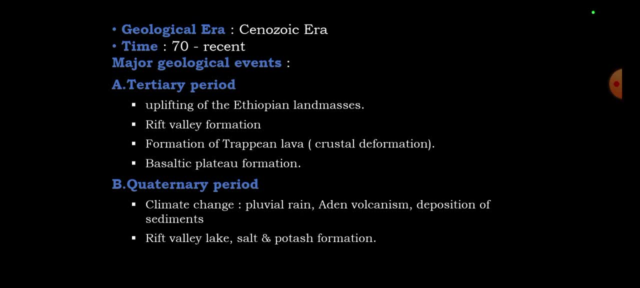 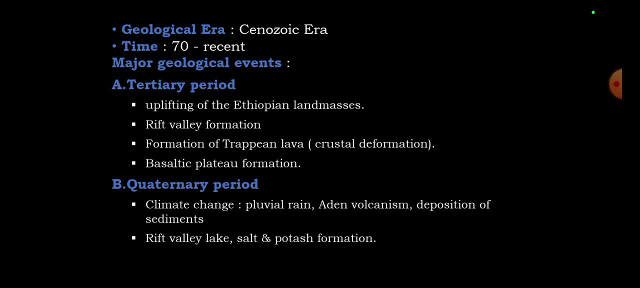 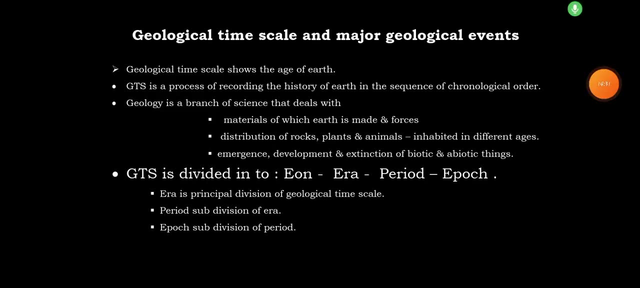 union channel like subscribe and do share madrigal you.